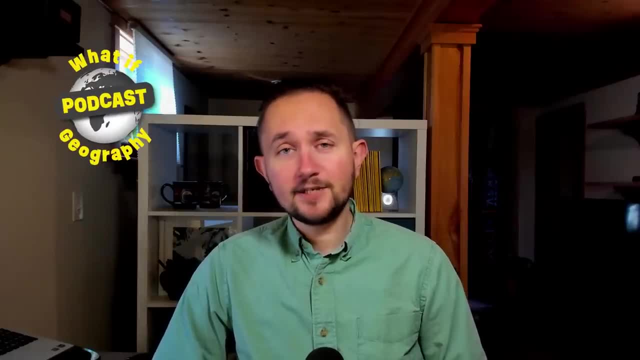 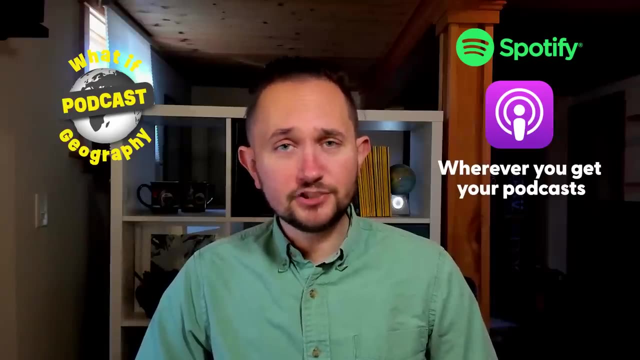 But before we get to today's episode, if you enjoy my content, be sure to check out the podcast that I co-host with Geography Professor Hunter Shobie. Each week, we bring you a fun-filled episode rooted in geography, And you can listen to every episode right here on YouTube, Apple Podcasts, Spotify. 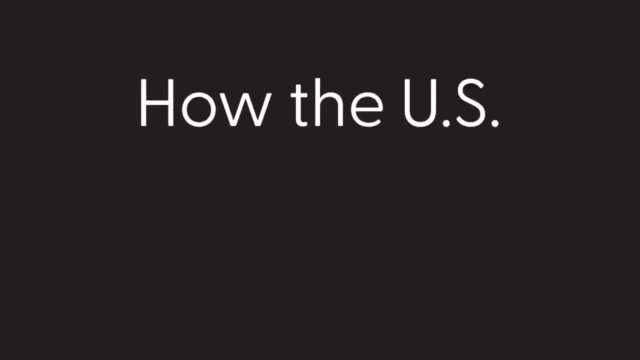 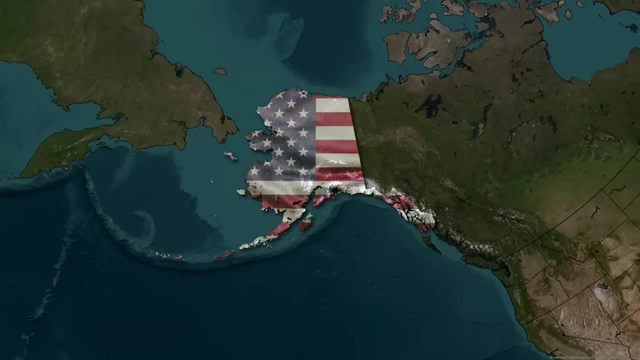 or wherever you get your podcasts. Alaska has kind of a long and winding history when it comes to how it ultimately ended up in the hands of the United States. While those of us who live in the United States take for granted that our largest state has always been there, the reality is that, were it not, 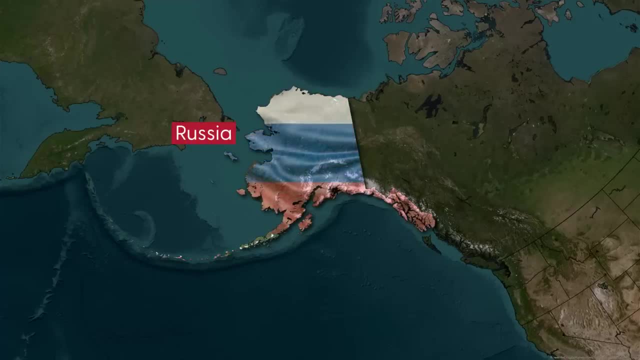 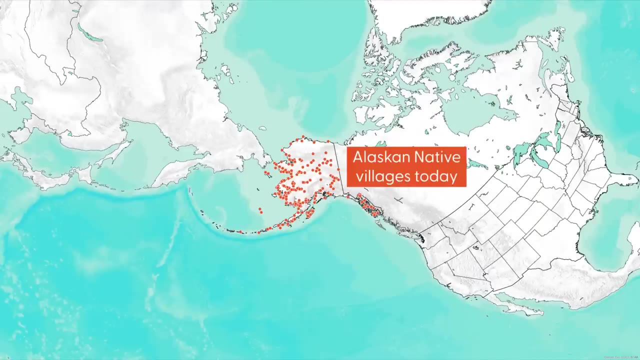 for a particular set of circumstances, Alaska would very likely remain with Russia or be a part of today. Alaska, of course, has always been inhabited by various indigenous tribes that still largely exist today, But during the Age of Exploration the first Europeans began making 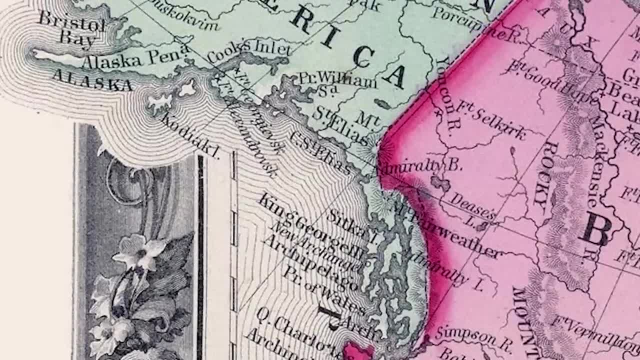 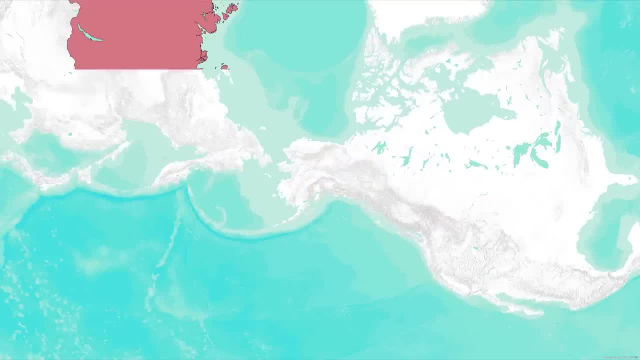 inroads into the general area. In fact, it's theorized that Russian explorers could have arrived on the shores of Alaska in the mid-1600s. Regardless of whether Russian explorers made it to Alaska that long ago, they certainly were the first to make it in the 1700s. This began. 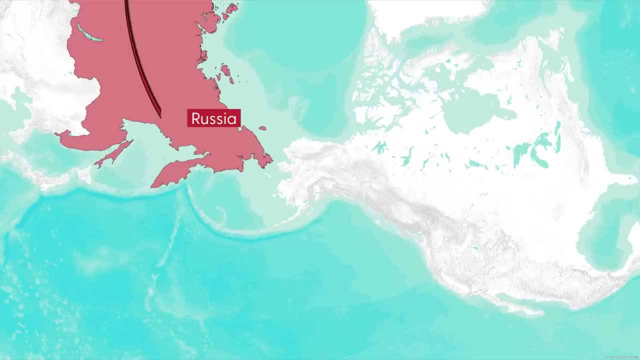 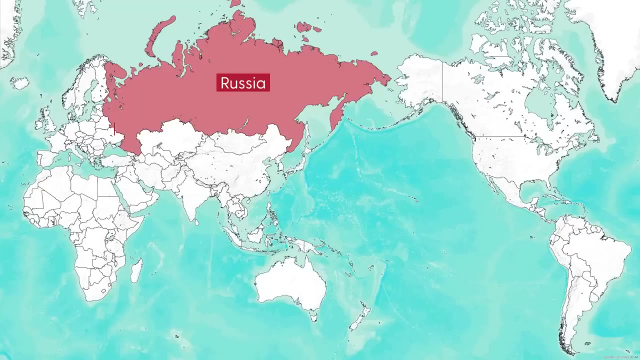 Russia's American colonial ambitions. The first full Russian settlement was founded in 1784, on Kodiak Island. Russia's colonies in Alaska, however, were never very profitable. Most of Russia's population centers were, and still are, based in the western part of their country. 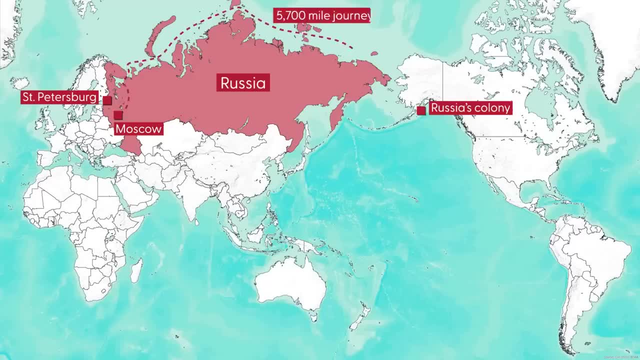 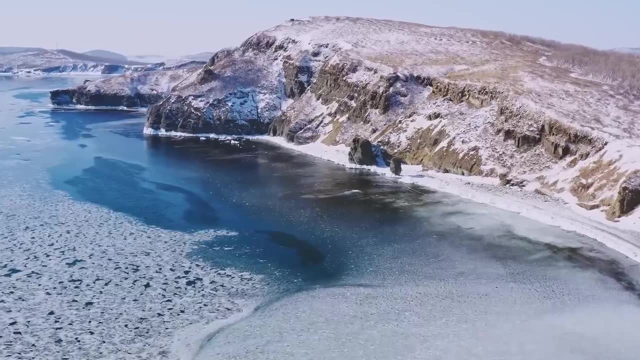 near Europe, which was very far away from the new Alaskan colonies, given the transportation technologies available at the time. And not only that, but Alaska was also very inhospitable. During the mid-1700s and 1800s, the world was far colder than it is today. 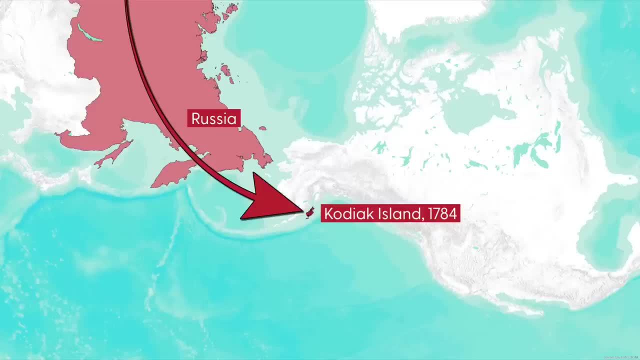 and this led to an Alaska that was much more difficult to live in. But Russia wasn't the only European power with eyes on Alaska at the time. The Spanish and British also believed that the area should belong to them. The Spanish held that the entire region was theirs, based on a 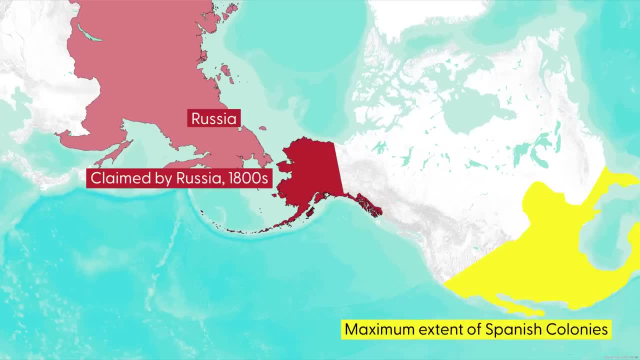 proclamation made in the 1400s, but no Spanish colonies or forts were ever founded in Alaska. Likewise, the British would establish a few trading colonies in the mid-1700s, but mostly focused their efforts on the rest of British Canada, including their ongoing dispute. 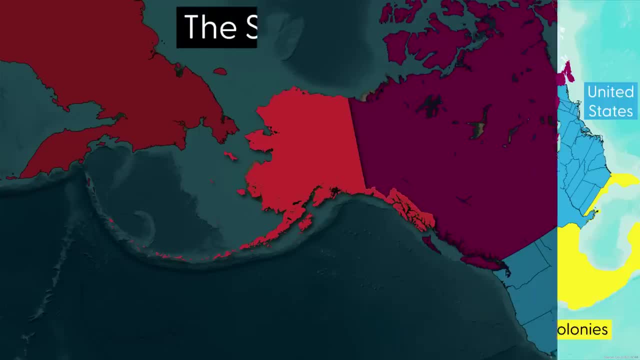 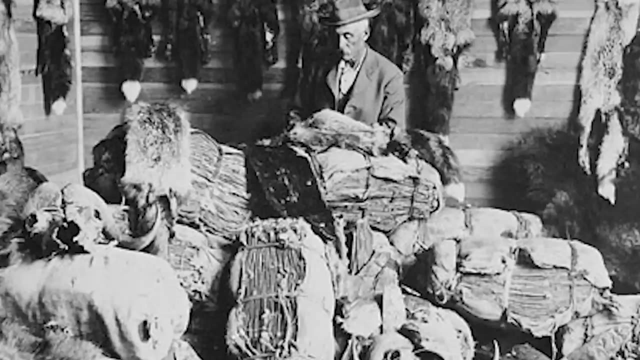 with the United States over the Oregon country. By the 1860s the Russian government was ready to abandon its colony in Alaska, but the British were not ready to do so. The British were not overhunting, severely reduced the fur-bearing animal population and competition from British. 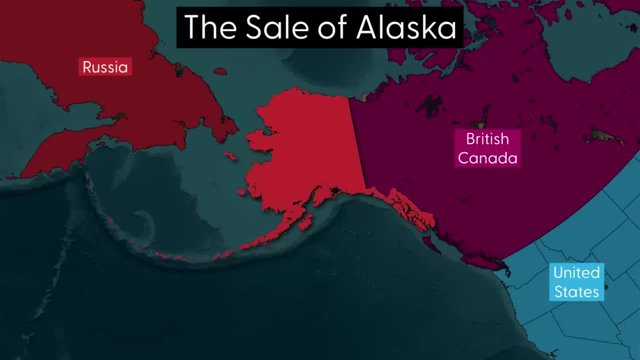 and Americans made it unprofitable for the Russian Empire. This, combined with the difficulties of supplying and protecting such a distant colony, reduced interest in the territory. Not least Russia at the time was feeling like the Alaska Territory would eventually fall into Britain's. 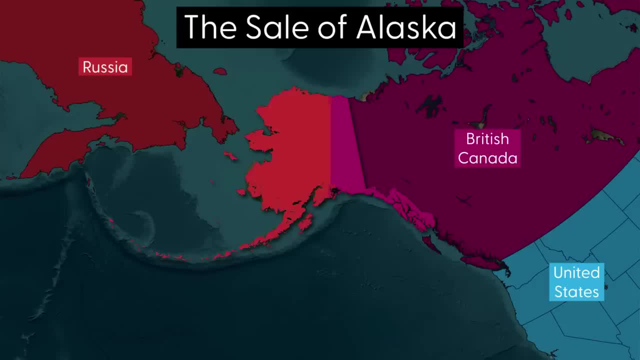 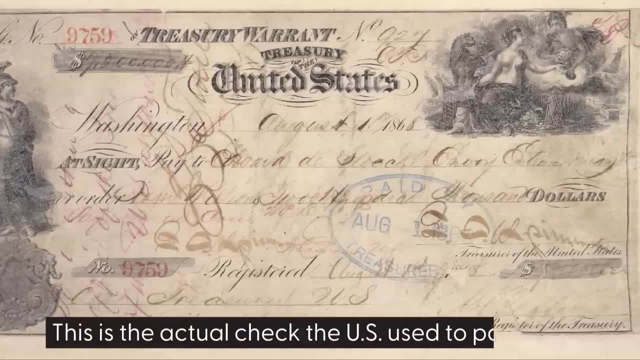 hands if they didn't do something. So they opted to sell the territory to the United States instead. In 1867, the United States and Russia formalized the sale of the Alaska Territory for a total of $7.2 million. Alaska as a US territory would exist as a military colony. 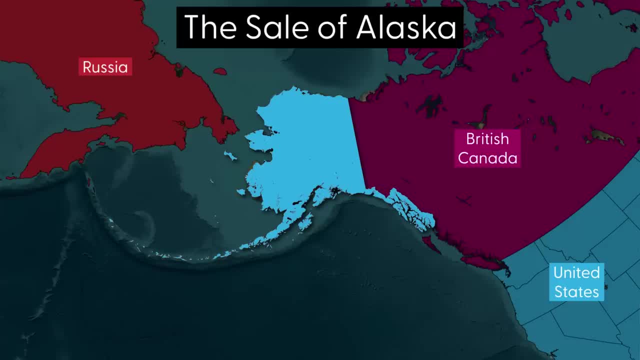 of sorts, with the military running the state between 1867 and 1884.. From then, the US president would appoint a governor to oversee the territory. Cities within Alaska were not even able to be formally incorporated until the year 1900, and it would take another 59 years. for Alaska to become a full state. with the passing of the Alaska Statehood Act, The United States bought Alaska at the low, low price of about $11, per square mile. That's an incredible deal, And while Alaska is still not very populated and 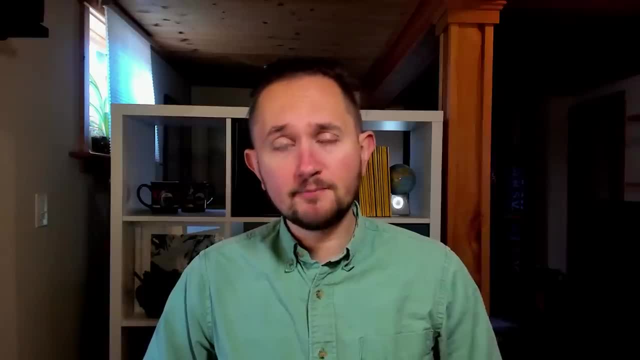 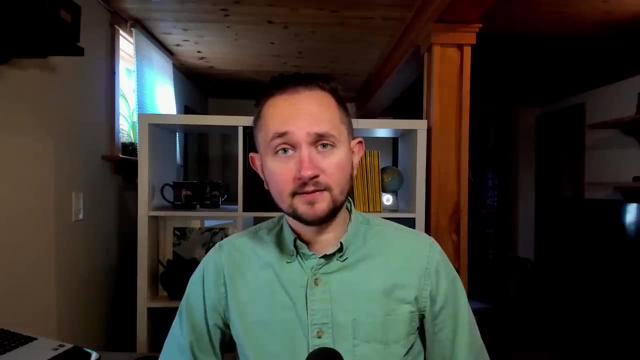 exists very far away from the rest of the United States, it's still incredibly important for the country as a whole. But before we get into exactly why Alaska is so important, if you're enjoying this video, hit that subscribe button. More fun geography videos are just a single click. 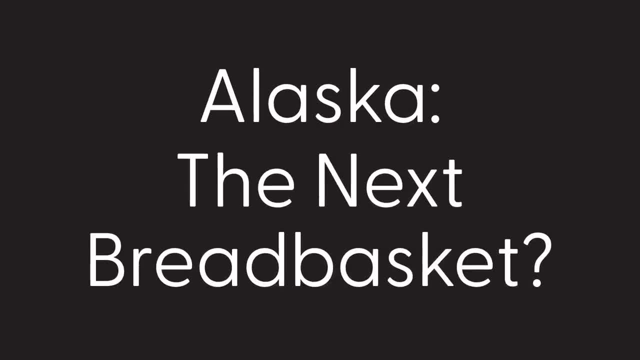 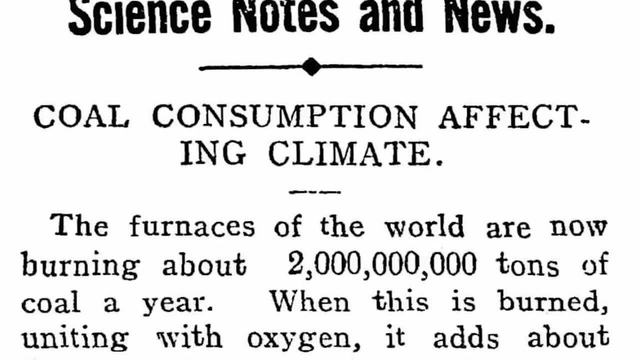 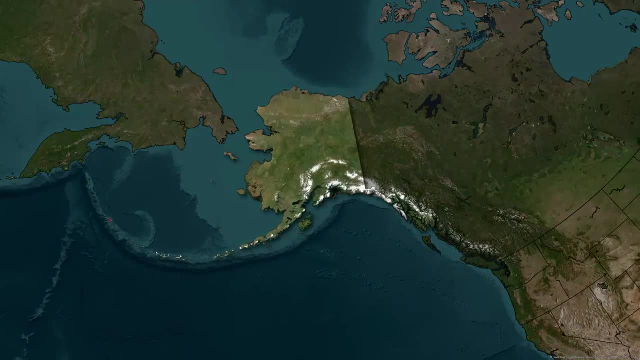 away, While scientists certainly weren't predicting the kind of rampant climate change we're beginning to experience today, though some scientists were saying it's not going to be as bad as we think it's going to be. it's going to be an incredibly wise investment in terms of future resource gathering, But that's not to say climate change. 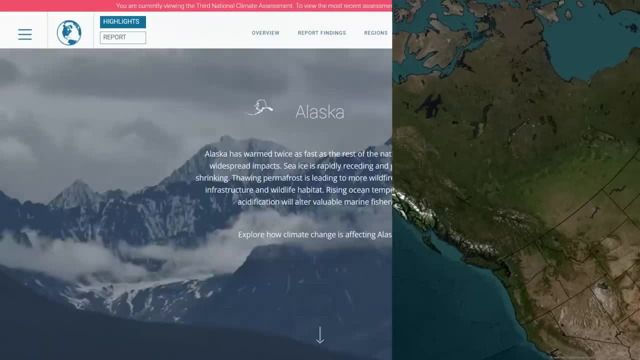 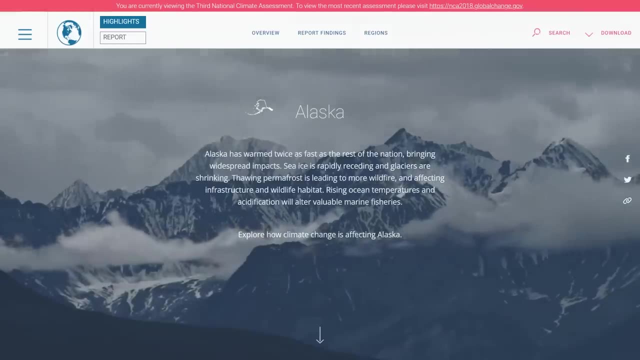 will be good for Alaska. Quite the contrary. According to the National Climate Assessment created by the US Global Change Research Program, Alaska is heating at a rate twice as fast as the rest of the United States. This has already caused widespread glacier melt. 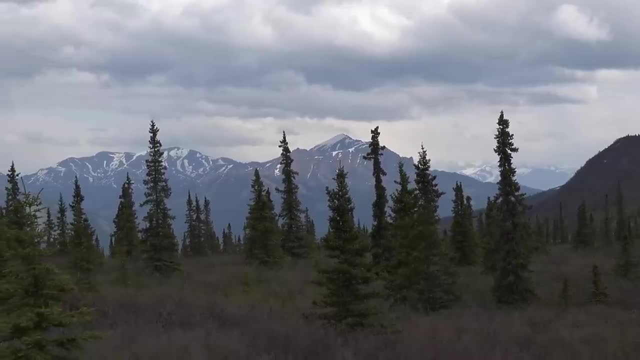 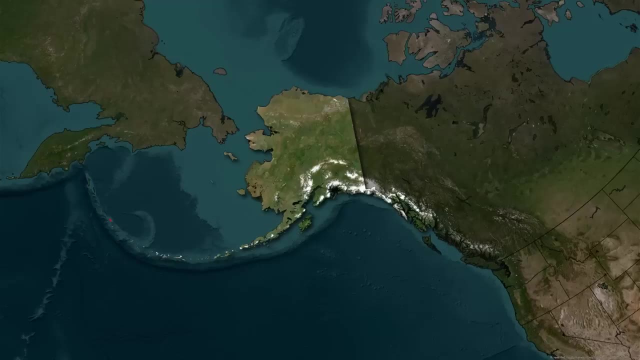 reduced sea ice, reduced permafrost- leading to the drunken forest effect- and, of course, an overall drier climate that leads to larger and more dangerous wildfires. But there are some potentially huge benefits to the United States at large if climate change were to cause serious disruption to the rest of the country. 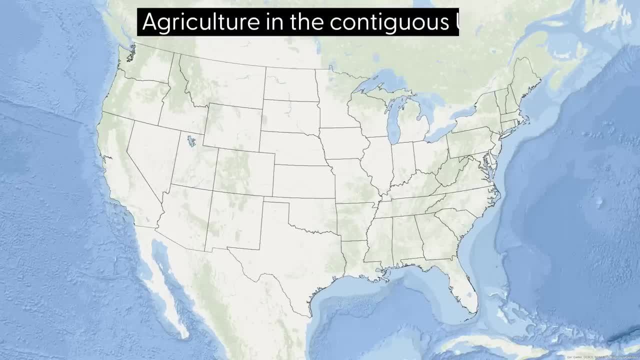 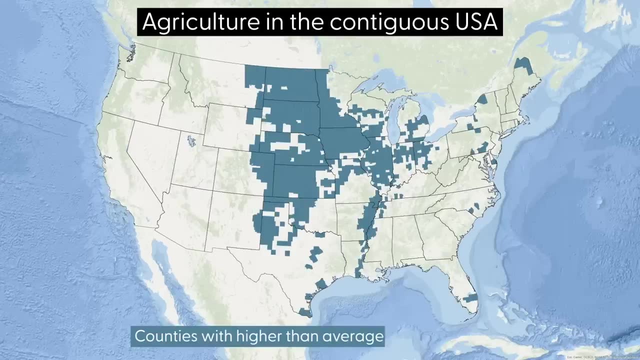 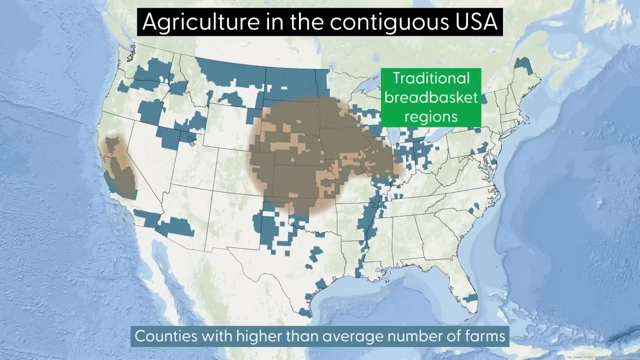 The biggest being agriculture. As it turns out, owning Alaska during the age of climate change could lead to a new breadbasket for the United States. Current climate change models are predicting that the traditional breadbasket regions of the country, such as the California Central Valley and the Midwest, will become drier, making growing a vast quantity of crops. 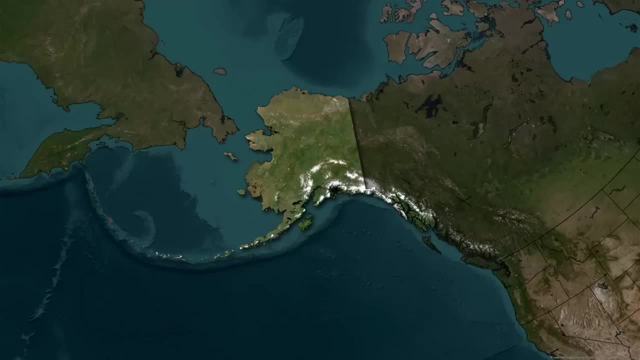 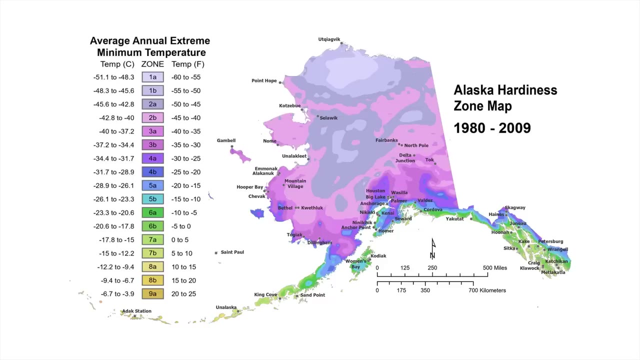 very challenging, But Alaska, a huge state already with quite a lot of water, could pose as a potential solution. Between now and the year 2100,, the amount of days Alaska is expected to be able to farm food will double. This means that food that normally wouldn't have been able to be grown in Alaska. 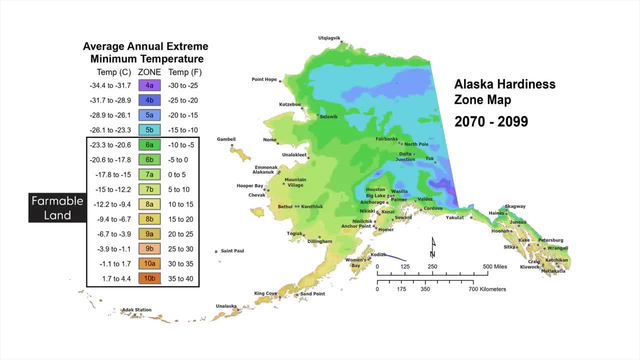 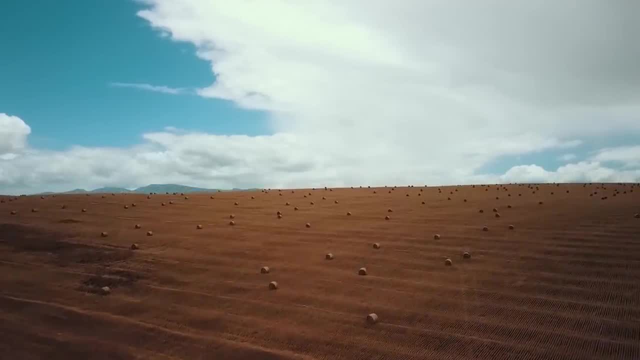 due to the amount of time required in warmer weather, will suddenly become much more viable. Grains such as barley and wheat could become a large agricultural product for Alaska, just as it becomes less viable in the south. And not only will the growing days double. 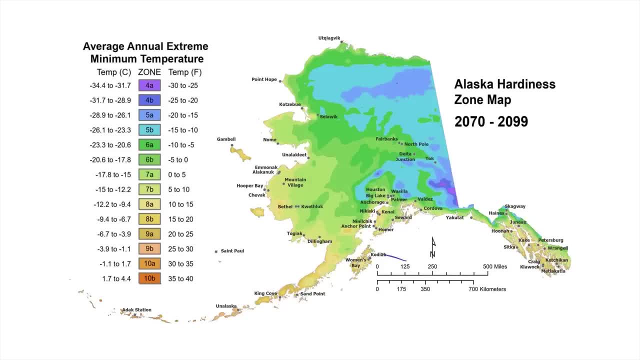 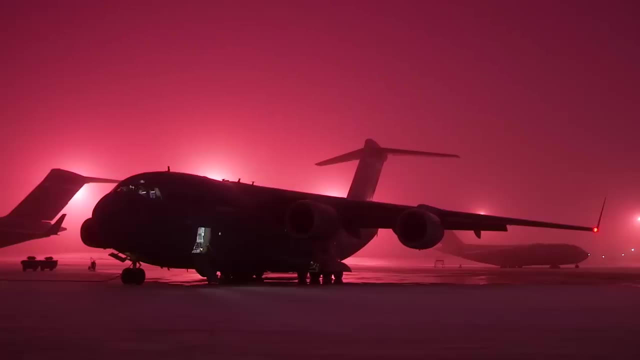 but the amount of land available to grow on will expand more than 100 times. Fairbanks, for example, can't grow much today, but over the next few decades it could become an agricultural hub, shipping food all across the world. Thankfully for Alaska, it's already in a very strategically opportune area for moving things around quickly. While food generation from Alaska will be very important for the United States in the future, Alaska is hugely important for the United States' strategic operations today. The whole state of Alaska and its biggest city of Anchorage are both located near the North Pole And because of this, despite what many maps would have us believe, Alaska is located very close to a number of the world's most important countries, including those that compete directly with the US. If we were to draw a straight line, the distance between Anchorage and Beijing is 3,970 miles, Moscow 4,342 miles, Tokyo 3,457 miles, and Berlin. 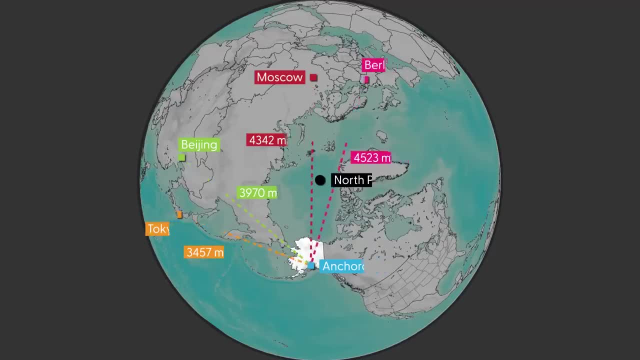 at 4,523 miles. To put this in perspective, the straight line distance from Washington DC to Moscow is nearly 4,900 miles. Los Angeles to Beijing is over 6,200 miles. Because of these shorter distances, the US military has a huge force stationed in Alaska year-round. 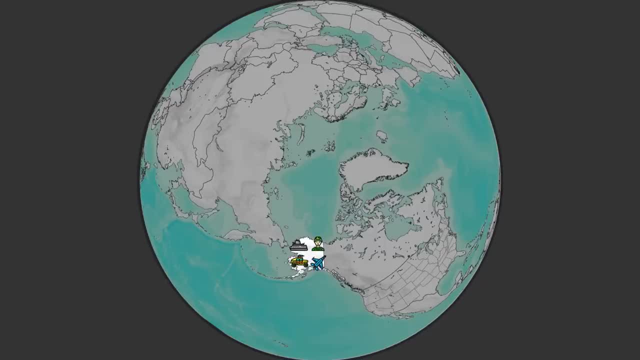 As you watch this video, over 22,000 Air Force, Army, Navy and Marine Corps personnel, along with 4,700 Guardsmen and Reservists, are operating within Alaska today, And with Alaska, it's very likely that the US military will be able to get to work with them. 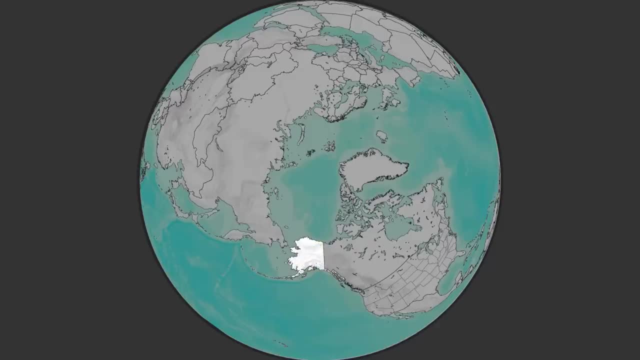 And with Alaska it's very likely that the US military will be able to get to work with them. strategic location: the US military can deploy almost anywhere in the Northern Hemisphere in very little time. But while Alaska is definitely important for military strategy, Alaska is also 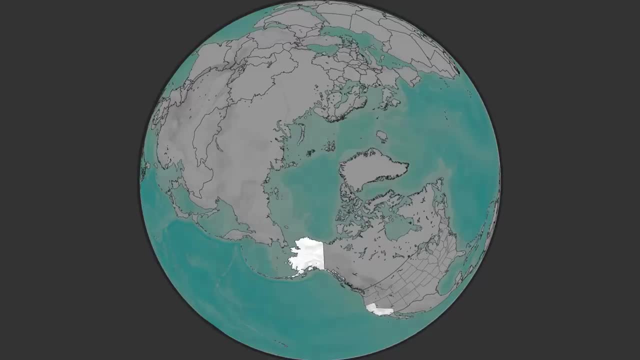 very important for consumer logistics For the same reasons as we previously covered. there exists a huge freight terminal for air cargo in Anchorage. According to the US Department of Transportation, over 1.6 million tons of freight flew through Alaska in 2021.. That's. 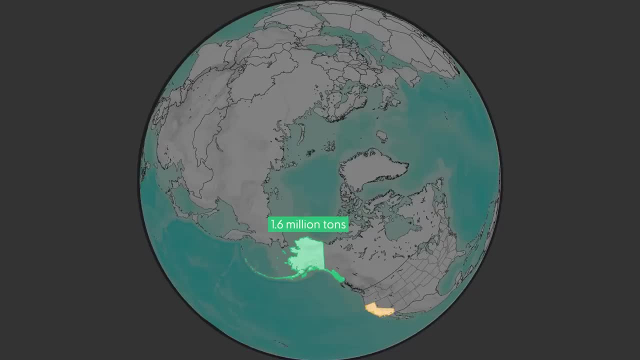 an incredible amount of freight. California, which has a population about 55 times larger than Alaska, had about 2.1 million tons of freight go through it. Bottom line shipping freight through Alaska cuts down on travel costs quite a bit And while air freight transportation 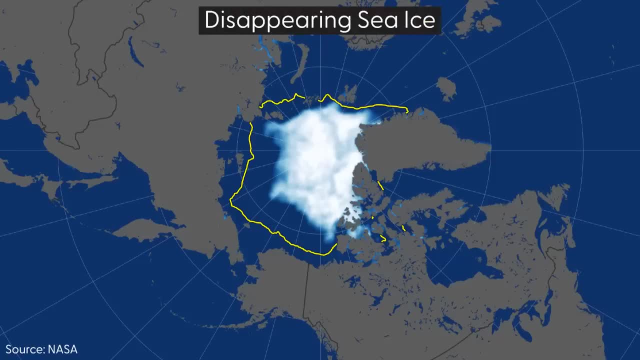 is incredibly important. receding ice in the Arctic Ocean will also yield new potential trade routes in international waters close to the North Pole. The prospect of a maritime link in the Arctic between Japan, China and the United States is growing and will only increase the strategic. 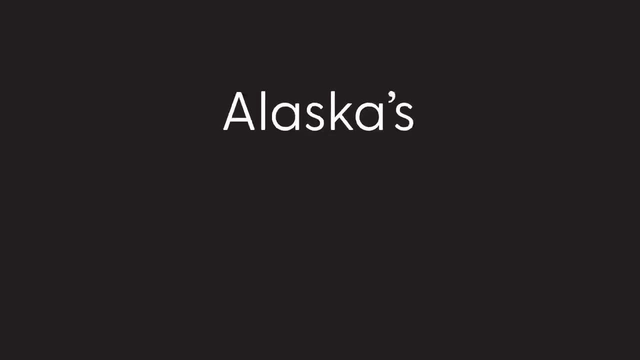 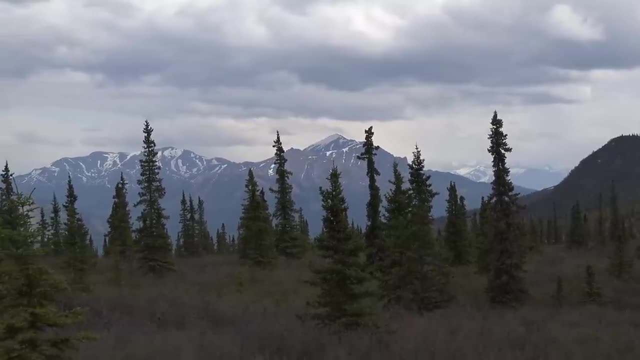 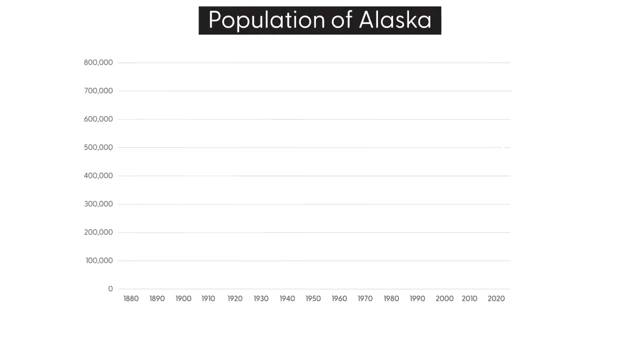 importance of Alaska to the United States. While Alaska is important for the United States in terms of military logistics and future agriculture, the state today is in a bit of a bad situation. Since 2010,, the state has suffered from rather anemic growth. In fact, the state is expected to lose population over the coming decades. 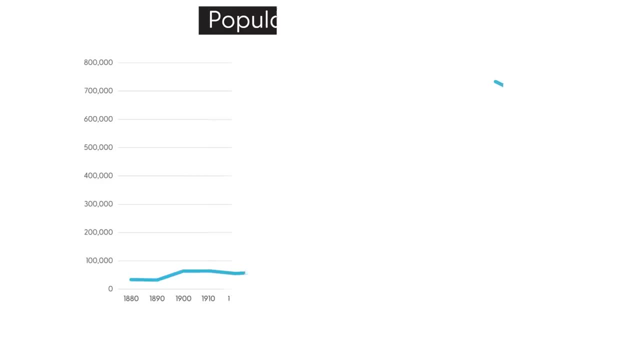 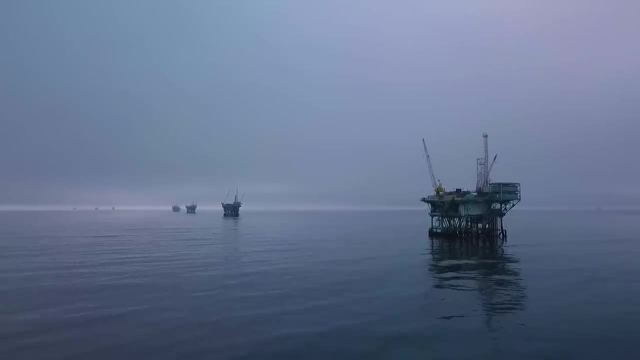 which is never something a state wants to see. Much of this lack of growth is due to the fact that the current economy of Alaska is incredibly dependent on natural resource development, the biggest of which is the state's oil industry, And, unfortunately for Alaska, 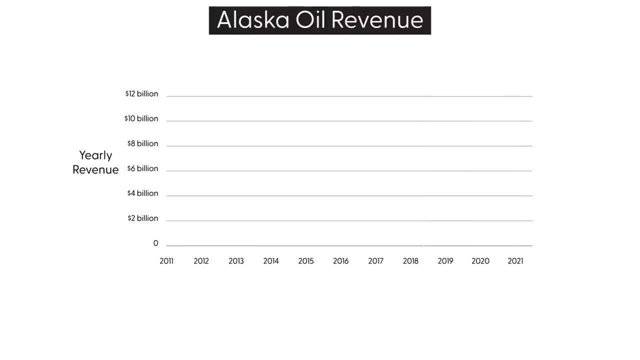 it's kind of running dry. According to recent state plans, the state's current intake of revenue from oil is about one-eighth as much as it was in 2012.. For a state with no sales tax, no income tax and very few taxes overall, this doesn't bode well for the state's solvency into. 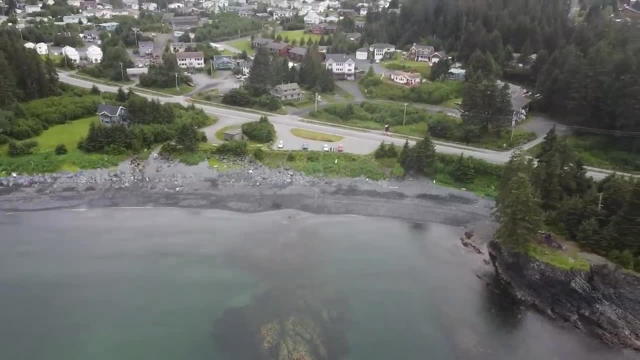 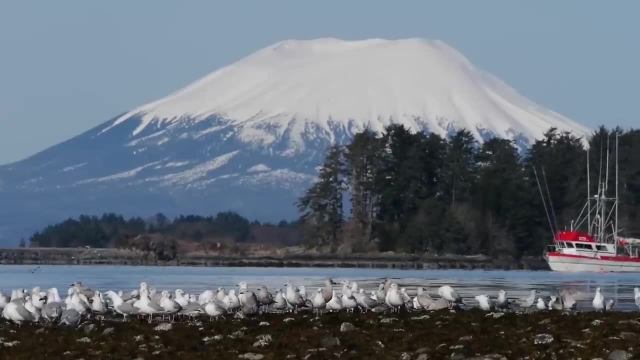 the future. This is compounded by the current system where the state of Alaska actually pays its current residents based on its expected income from the oil industry. So not only are Alaskans not accustomed to paying taxes, but they actually expect money from their state every year. 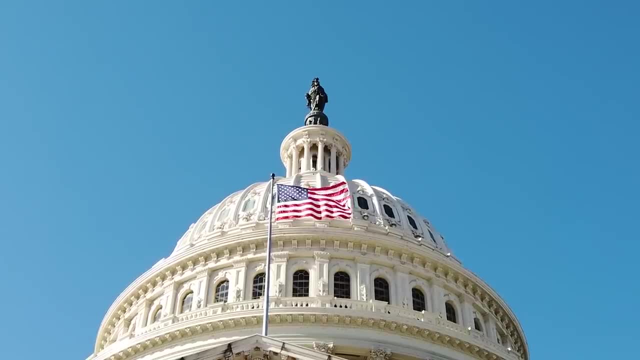 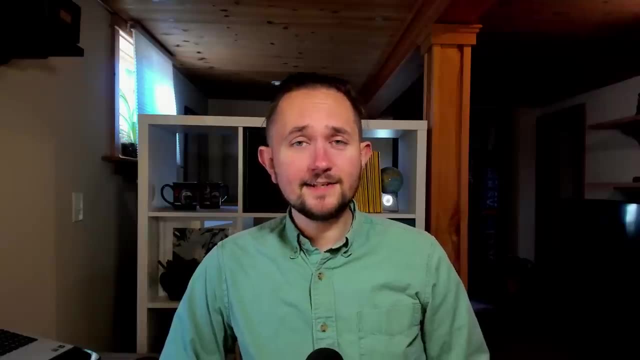 Luckily for Alaska, the state is just so incredibly important to the US that if it were to get into any serious trouble, Uncle Sam would absolutely make sure it stays afloat. Alaska is the United States' secret superpower. While the state is not a secret, of course, the power and importance of the state 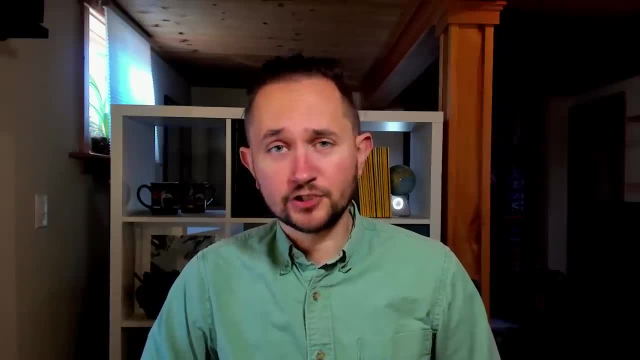 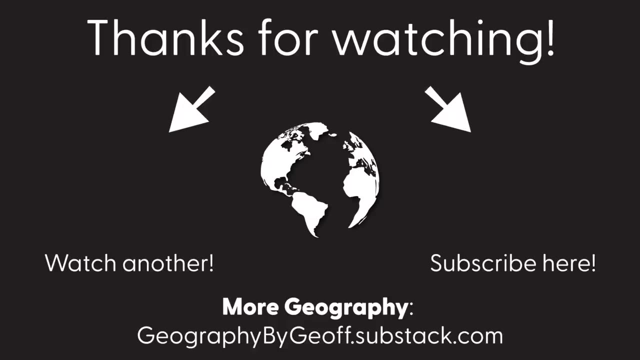 will help solidify America's security and dominance well into the future, And for those of us living in the United States, we should all feel lucky that the US owns it and not Russia. I hope you enjoyed learning a bit more about Alaska's importance to the United States, If you did. 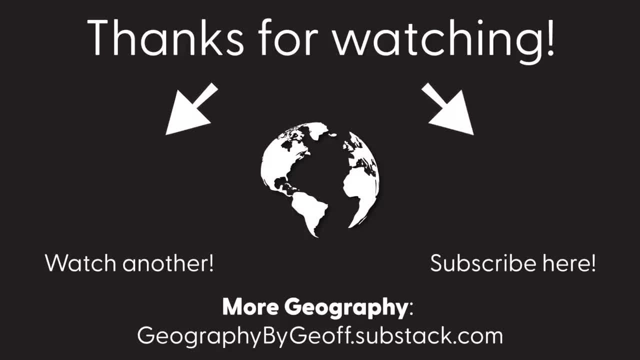 subscribe to my channel And if you want to watch more of my videos, you can do so here. Thanks for watching. See you next time.